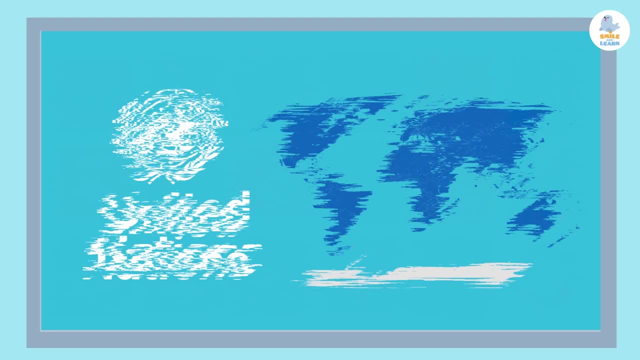 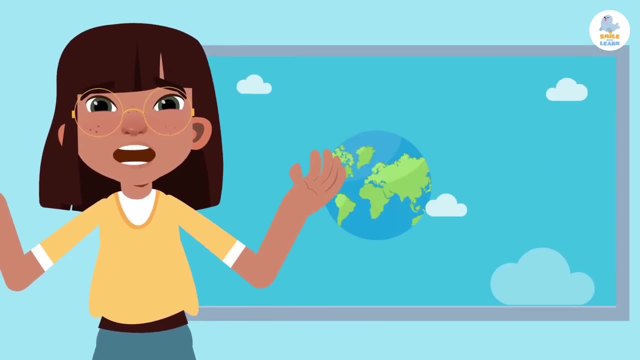 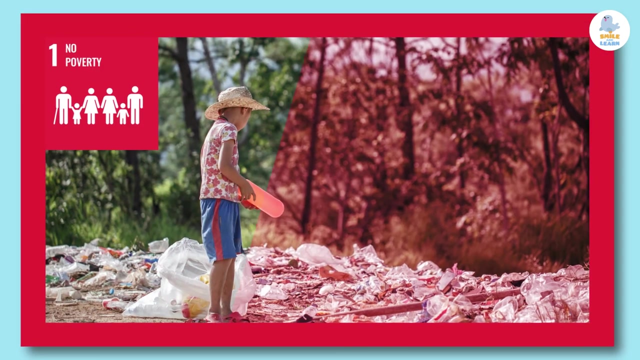 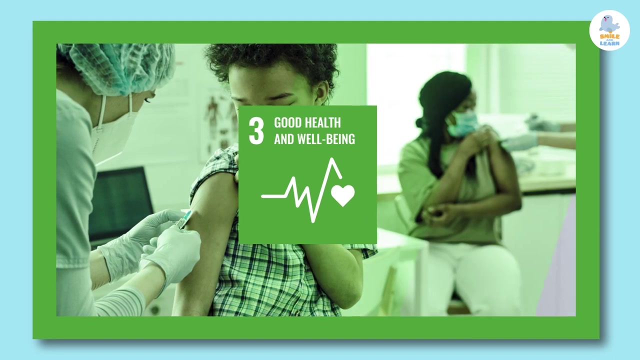 countries. The goal is to eradicate poverty, protect the planet and ensure prosperity for all. Let's see what they are. Number one: no poverty. Number two: zero hunger. Number three: good health and well-being. Number four: quality education. 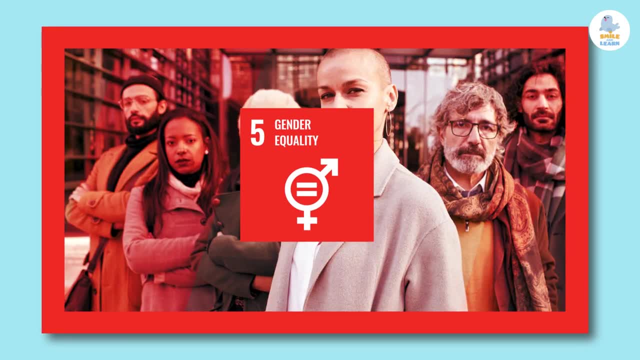 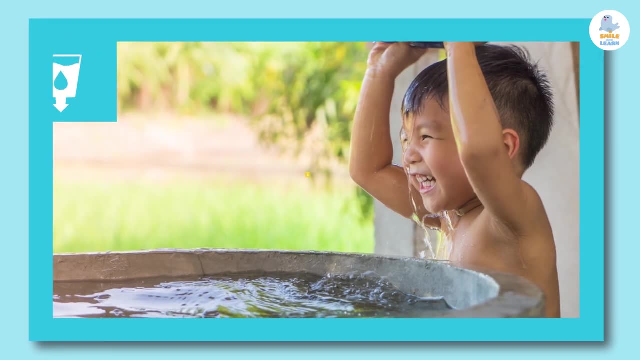 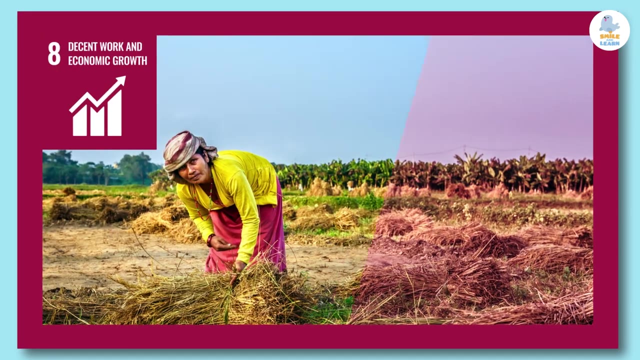 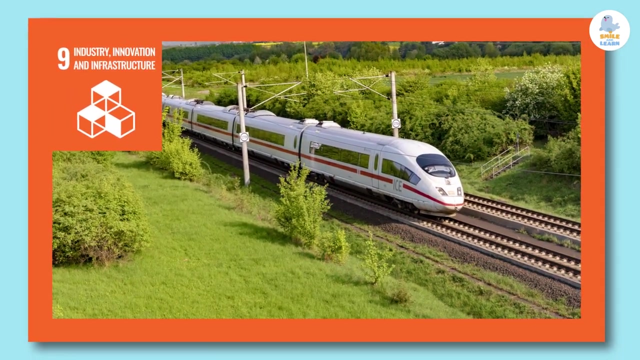 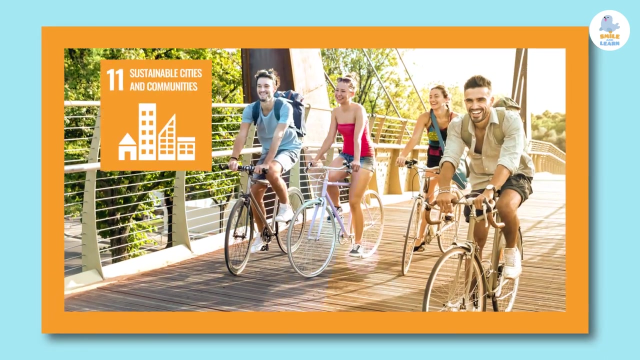 Number five: gender equality. Number six: clean water and sanitation. Number seven: affordable and clean energy- Number eight: decent work and economic growth- Number nine: industry, innovation and infrastructure. Number ten: reduced inequalities- Number ten: economic growth- Number 11, sustainable cities and communities- Number 12, responsible consumption. 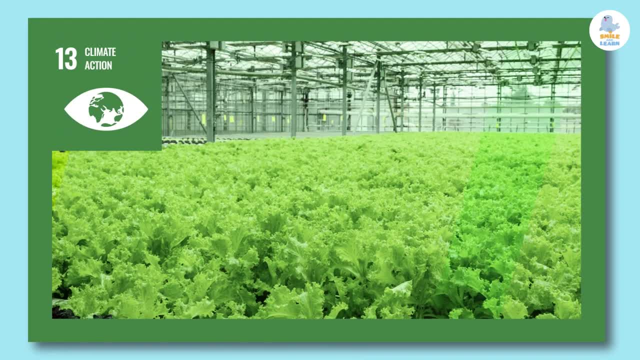 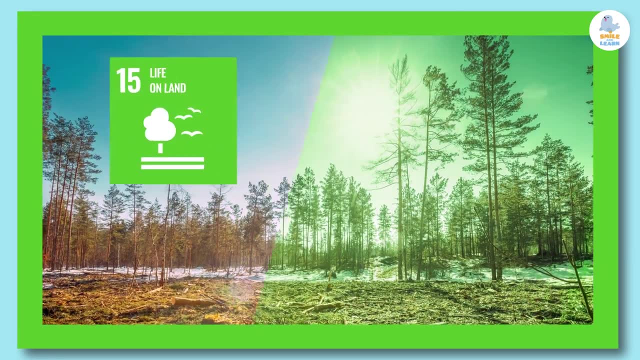 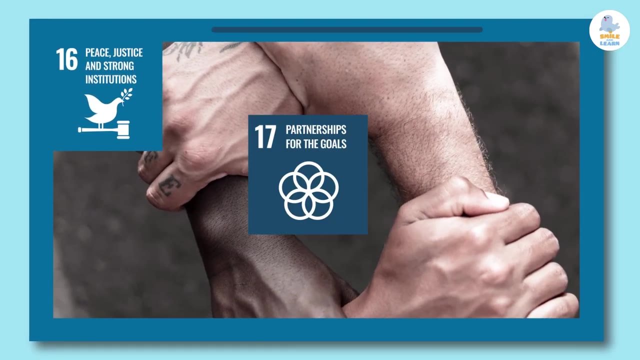 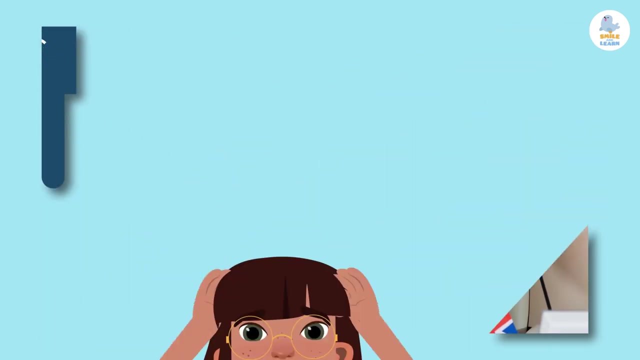 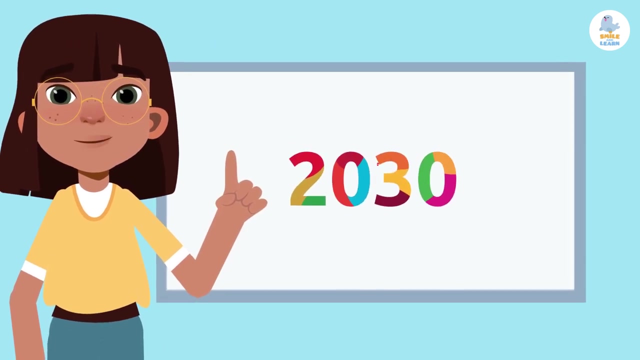 and production- Number 13,. climate action: Number 14,. life below water: Number 15,. life on land- Number 16,. peace, justice and strong institutions- Number 17,. partnerships for the goals: Wow, that's a lot. Each goal has specific targets to reach by year 2030.. To achieve? 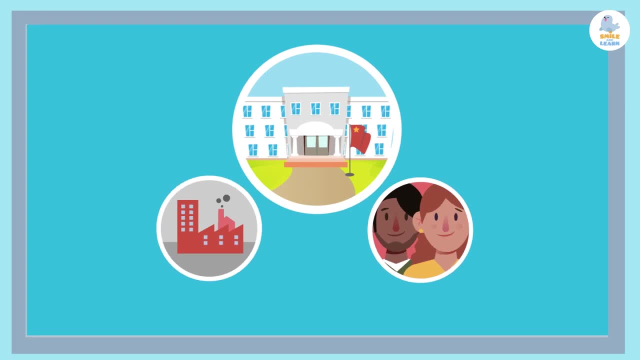 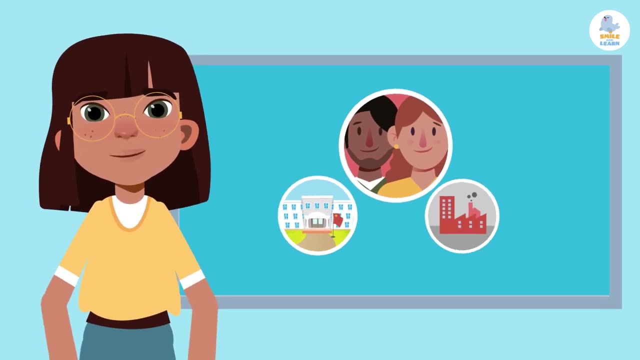 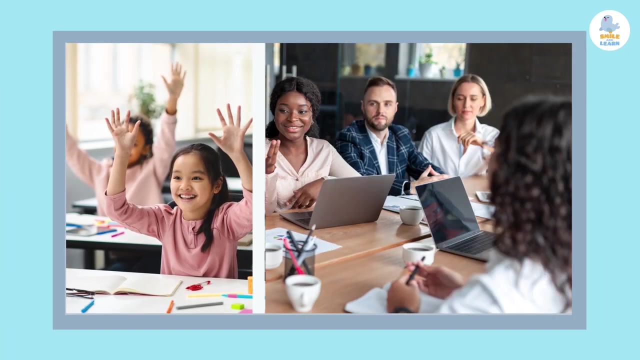 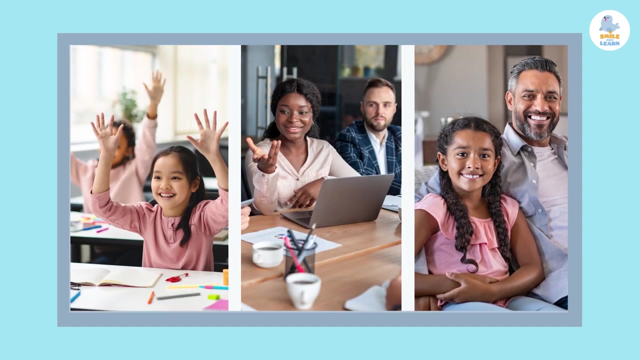 these goals. we all have to do our part: Governments, businesses and society too. In other words, each and every one of us. And how can we incorporate these objectives into our daily lives? Well, we should try to live in a more sustainable way, at school, work and home, For example. 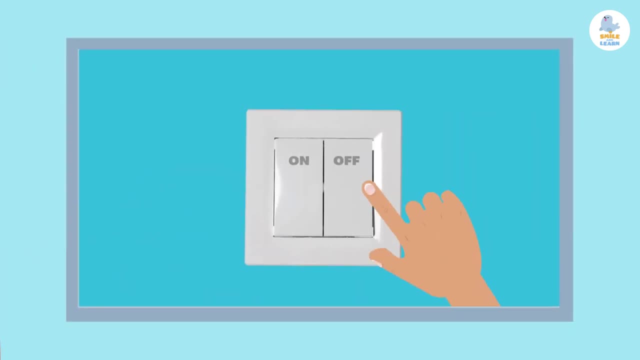 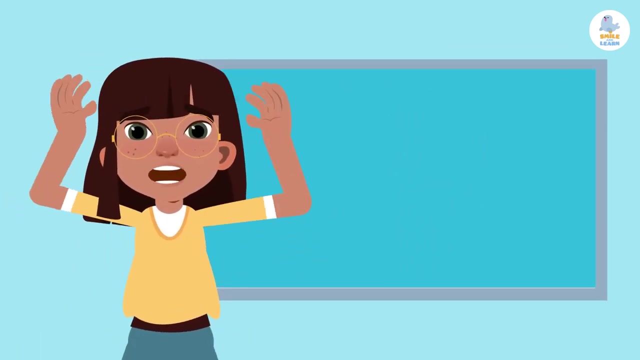 by improving our consumption habits, saving energy or caring for the flora and fauna. Don't worry if you don't know where to start. It happened to me too. Luckily, the UN made a very easy guide called Saving The World. Save The World.